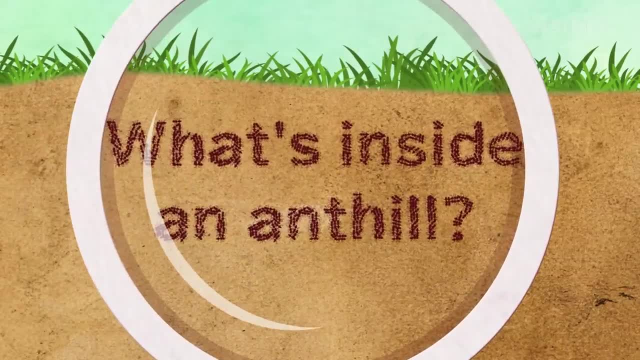 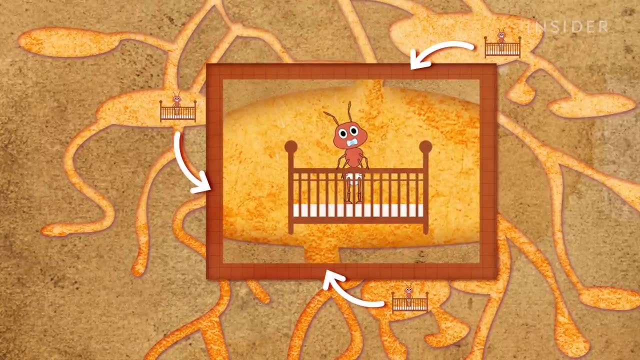 So let's take a closer look at what's inside an ant hill. The mound is really the top of an enormous underground structure, the nest, which is basically a giant nursery, a nice, cozy place to raise babies, A lot of babies. 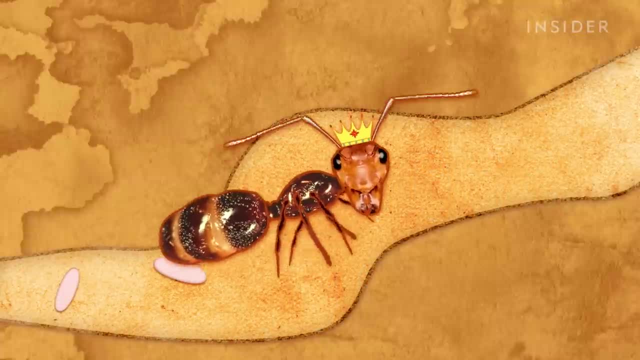 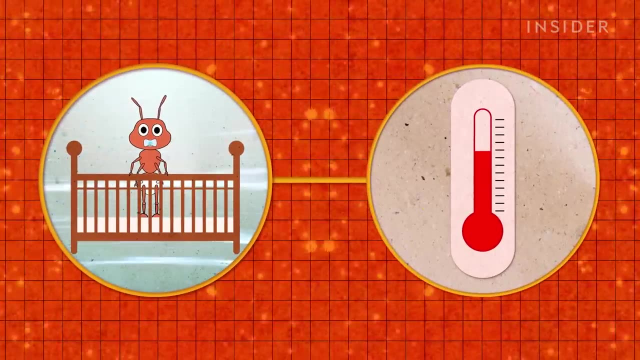 Their mother, the queen, roams around the nest while laying 1,500 eggs a day. Now, all those baby ants need to live in a narrow temperature range to grow, So that nest sports temperature-controlled rooms, and it does so without the help of an AC unit. 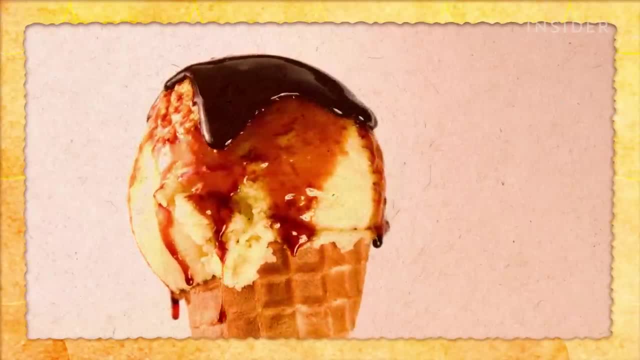 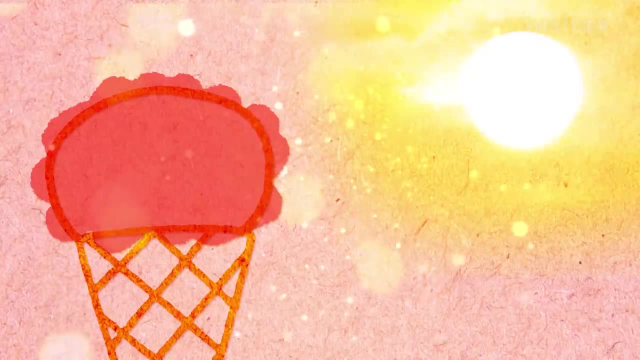 The secret is in the design. The nest is arranged like an ice cream cone. At the top you have the mound, the ice cream, as it were. Because it's above the surface, it warms from the heat of the sun. 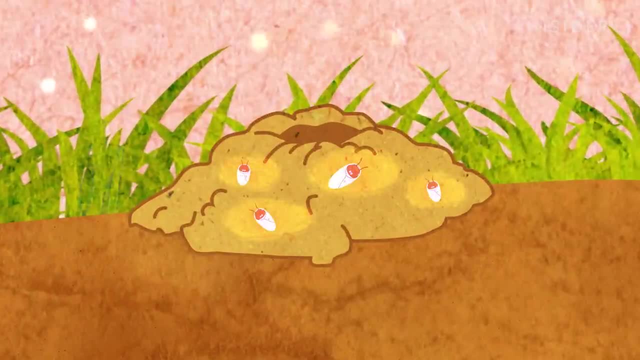 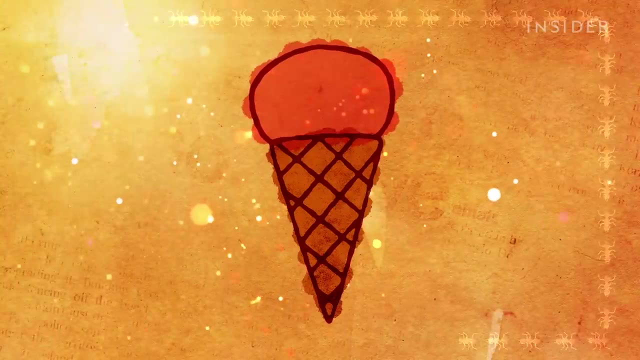 So the babies can snuggle up in toasty chambers networked throughout the mound, But they can't stay there all day or they'd get too hot. That's where the cone- part of the ice cream cone- comes in. The mound is connected to several vertical shafts that plunge up to two meters beneath the ground. 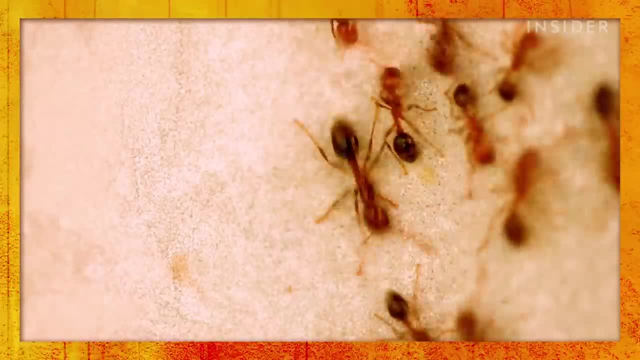 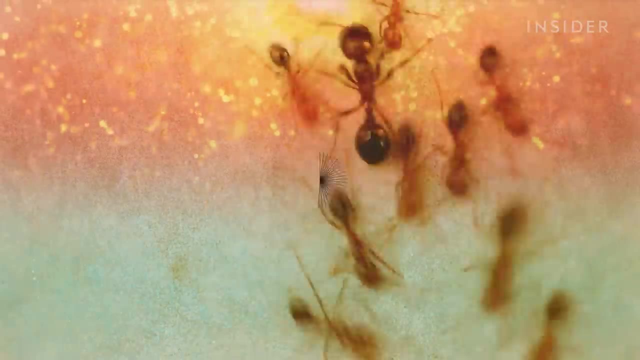 That's taller than most humans. Throughout the day, adult ants ferry. They carry the babies up and down the shafts, chasing that perfect temperature for their young charges. The nest also sports dozens of tapering tunnels that branch off from these main shafts. 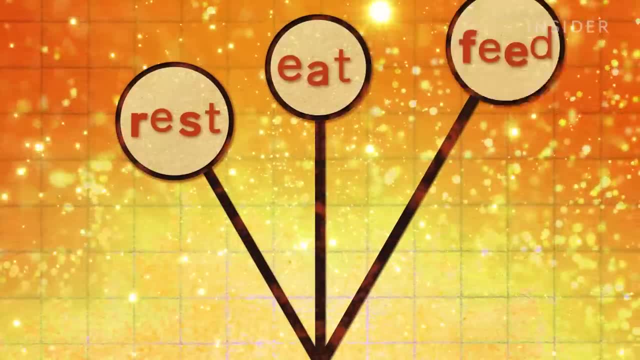 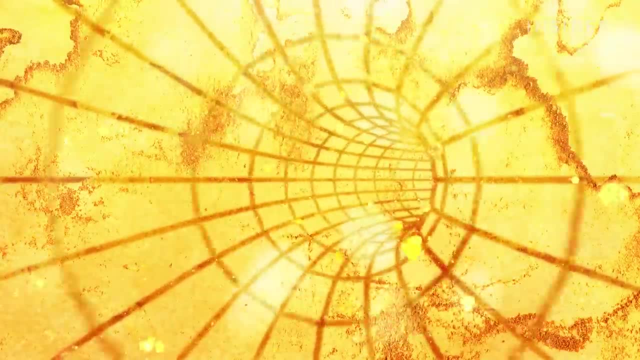 These connect to small chambers where the ants rest, eat and feed the babies until it's time to move the little ones once again. Now there's one more type of tunnel inside the nest, but only a few ants ever use it. You see, someone needs to find food for the rest of the colony. 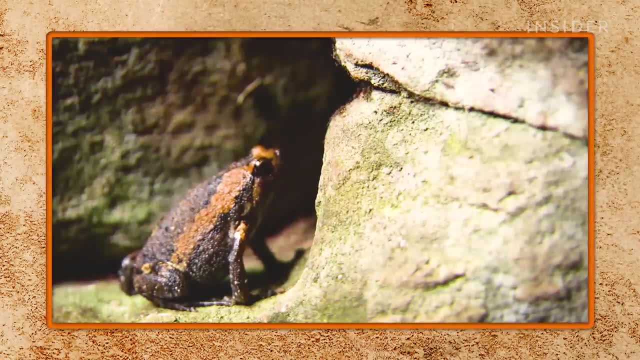 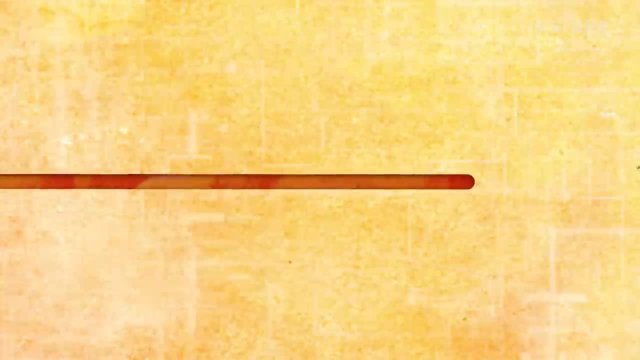 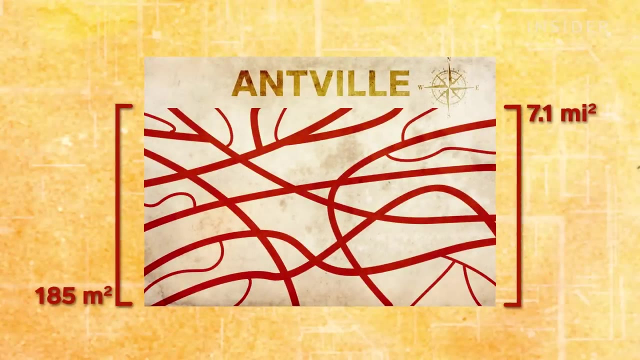 But running around outside the nest is not easy. That's where forager tunnels come in. These are a couple of horizontal passages buried just a few centimeters from the surface, But they run throughout the entire territory, which can cover up to 185 square meters of land. 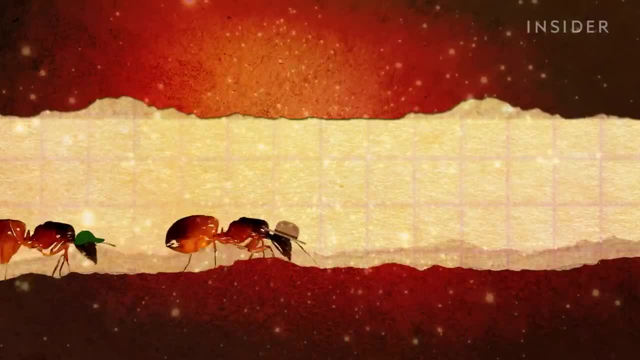 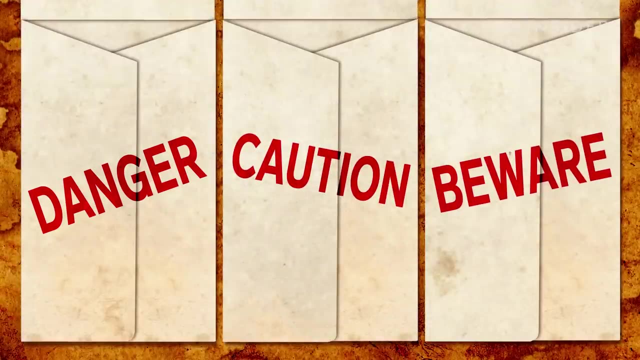 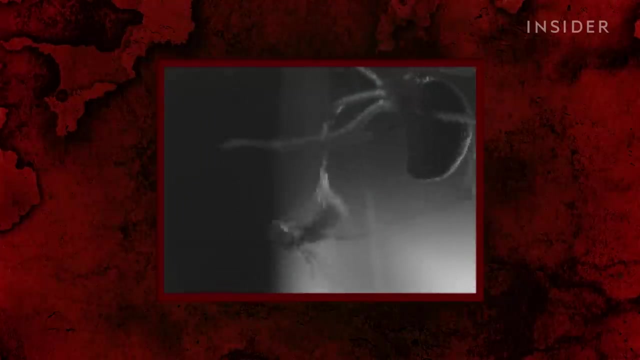 By scurrying through these passageways. the scouts can stay underground as long as possible, But unfortunately the nest and all its roads can't protect the ants from every threat. It turns out all sorts of critters sneak inside, And while many of them are actually harmless, others are horrible houseguests. For example, beetles burrow into the nest and devour the eggs and larvae. But invaders aren't the only threat to the colony. Occasionally, clueless humans or major floods disturb the nest, And when that happens, the fire ants have only one option.